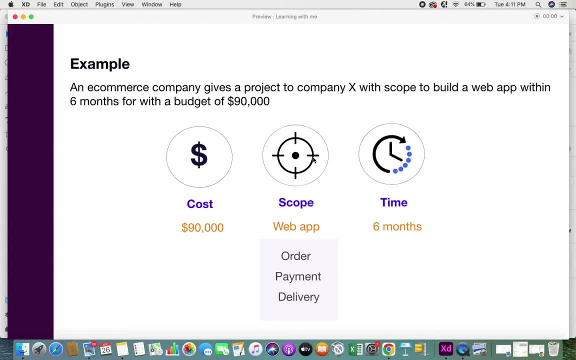 So, if you see, here we have three constraints, which is cost, scope and time. So we see that the scope is to build a web application and the features or the modules are order, payments and delivery, And the time is six months and the cost is about $90,000.. So now, with these three constraints, let us see different scenarios as to, whenever one constraint is altered, how the other two get affected. So, when you take the first scenario, 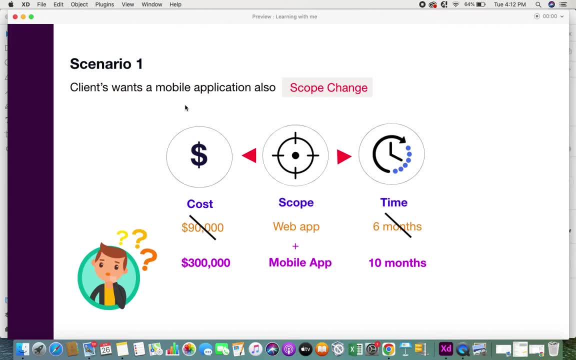 the client now wants a mobile application also. So if you see here there is a change in scope, Okay. so because of this scope change in previously it was just a web app but now it's a mobile application. So now the project managers they need to check and see if this scope change is going to affect the other two. Definitely it will affect the other two constraints. So, since this is something else that's added to the scope, definitely it will affect the cost. 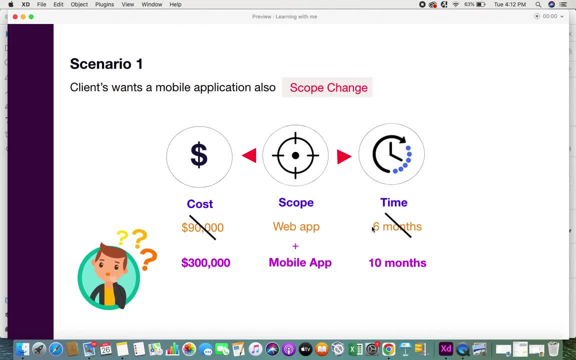 And the time. So what was able to be completed in six months, now it will require 10 months timeline And also, of course, cost will increase from the estimation that the project manager has put is from $90,000 to $300,000. Because it's the cost comprises of the various resources that are involved. Of course, you need to pay the people who are developing the app. you need to pay for other resources. 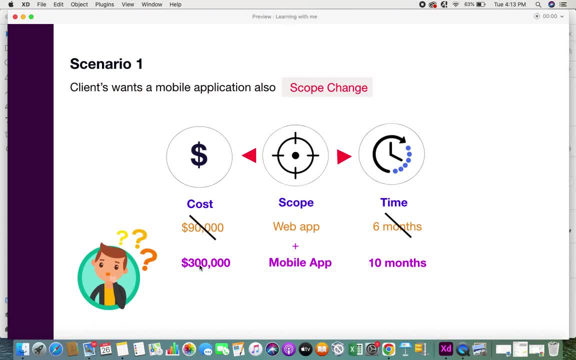 So, taking all that into consideration, there is also a alteration in the cost constraint. So this is about the scope change. The next scenario is: the client wants the project in six months. Okay, so now here there is a time change. So when there is a time change, he said so. the client says that instead of 10 months, they want it within six months. So of course, the project team will say that they will not be able to complete the scope over the other two. 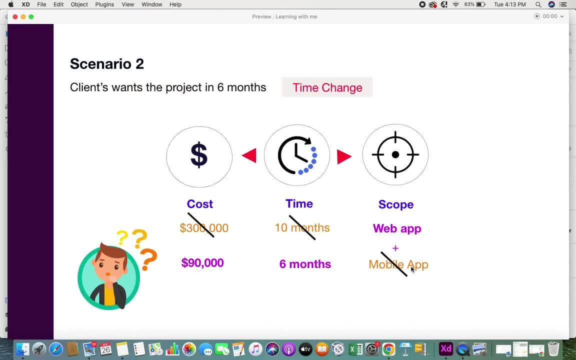 Items in the scope. So you have the web application plus mobile app. So since the time is reduced, it's going to affect the scope and the team comes up with an alternative saying that only the web application can be completed in six months. And when you see how this affects the cost side is since there is a particular module not being built, that's the mobile application side of it. the cost is also reduced, If you notice, sometimes if additional functionalities are added. 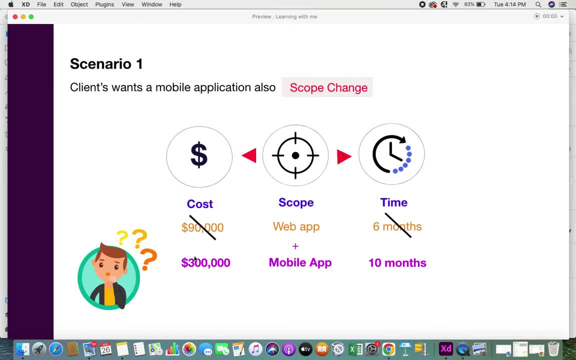 in the previous case, cost can increase also. So the third scenario is the client's budget is now only 60,000.. Okay, so because of some reasons, the client says that they have a very low budget, So at that time there is a cost change. So with this cost change- definitely they will- the team also will have to plan accordingly So as to how many people they can put onto the team in order to develop the app. 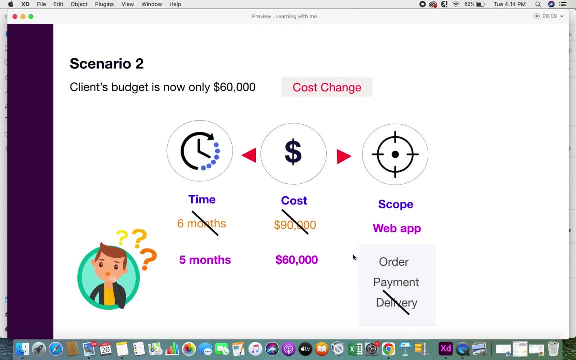 E-commerce application. So with that particular cost, it's estimated that the team will be able only to complete the web application with the order and payment module. And when you see the time, since it's some, the delivery module is not going to be, you know, worked on in that particular duration for that particular project. the time also may get altered to from six months to five months. So because of the change in cost, the scope and time now gets altered. 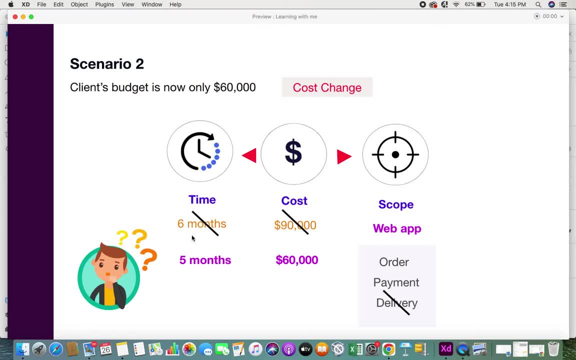 So this is the example of how, whenever a constraint is updated, it affects the other two constraints also. So this, the triple triangle, or the triangle constraints of a project, is very helpful when you need to, you know, plan for a project. It acts as a very good planner and a guideline. Okay, And there should always be a perfect balance between these three constraints: the time, cost and scope. Else, it's going to create a little bit of a chaos in the project. 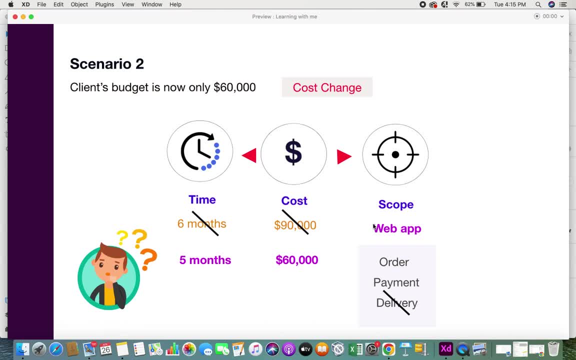 So that's what project managers always keep tracking and see. So I hope that you got some information on what is a triple triangle, a golden triangle or triangle, constraints of project management. So if you found this helpful and useful, please do give this a thumbs up. If you haven't subscribed, please do subscribe to this channel and also do share your feedback and share it to your friends. Thank you.